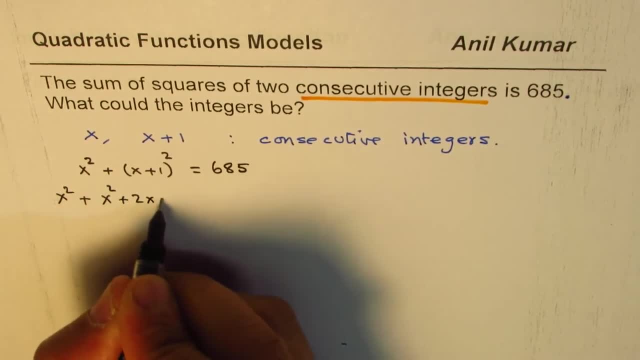 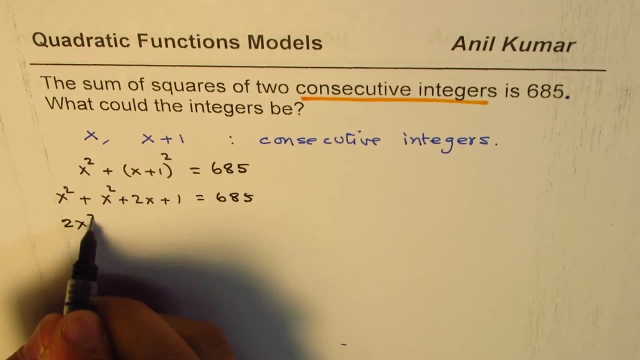 plus, when you open this up, you get x squared plus 2x plus 1 equals to 685.. Bringing 685 to the left, combine these two terms: 2x squared plus 2x. Bringing this here, we get minus 685 equals to 0.. Combining again: 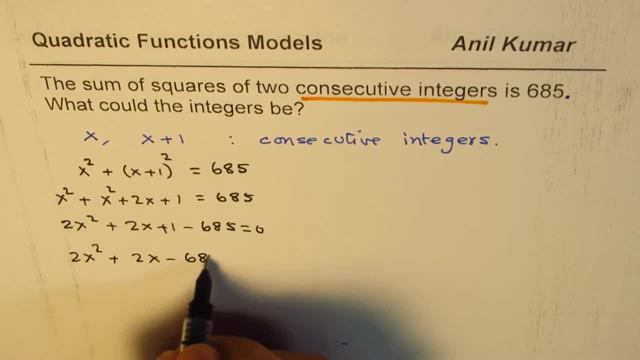 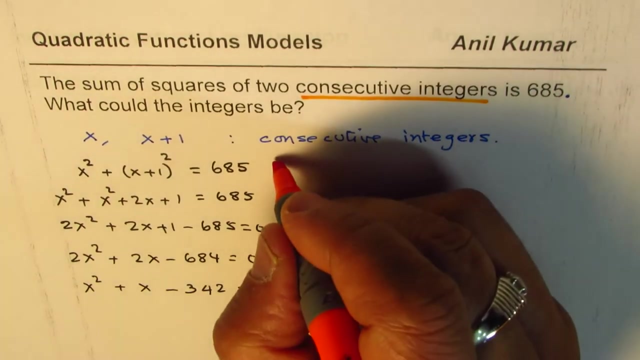 2x squared plus 2x minus 684, equals 0.. You can divide by 2, right? So you get x squared plus x minus half of this, 342.. Equal to 0.. Now, at this stage, you could use product and sum, or you could use quadratic. 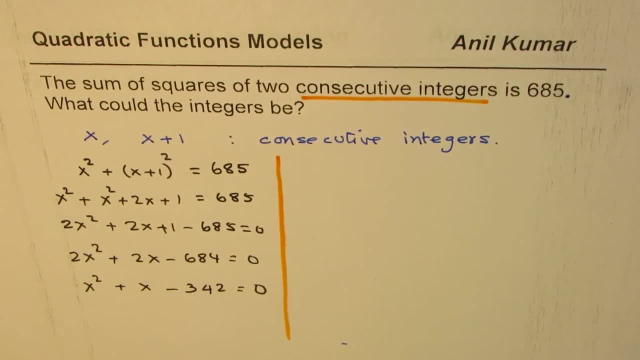 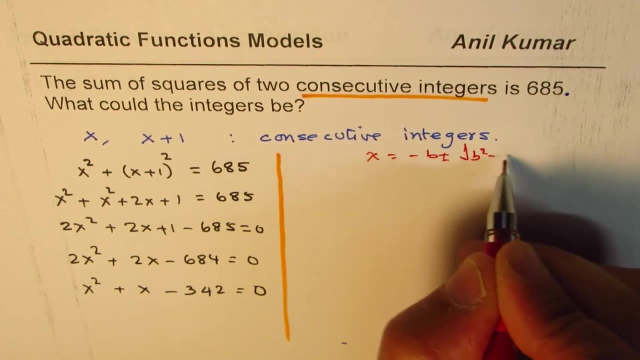 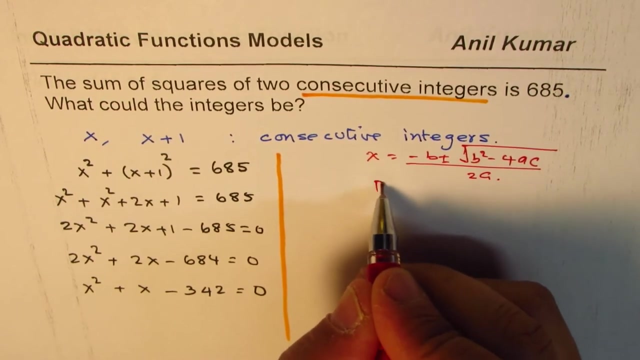 formula right Factor and solve or use quadratic formula. So the quadratic formula will be of this form. You can say: x equals to minus b plus minus square root of b squared minus 4ac. divide by 2a And product and sum method could be: you're looking for a product of minus 342.. 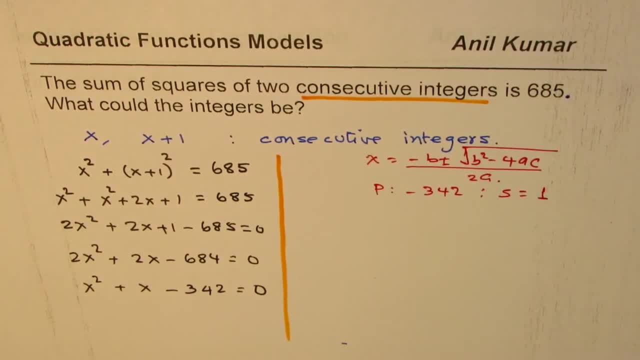 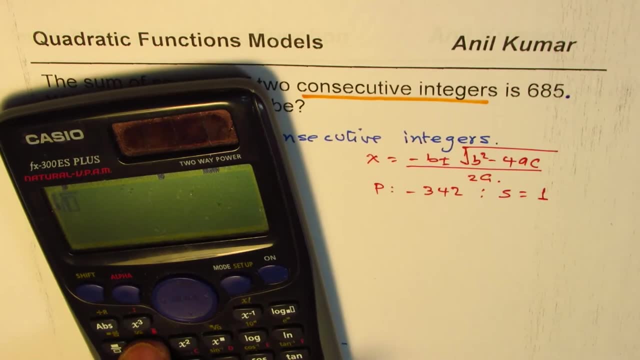 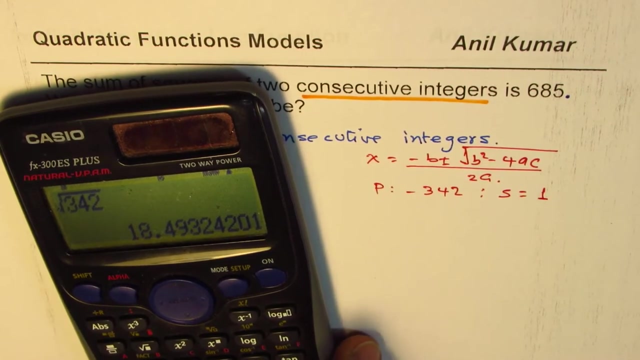 And product and sum of 1, correct. So that means these two numbers are very close, very, very close. Very close numbers you can always get by kind of square root right? So if I do square root of 342 and approximate this to a decimal place, it is somewhere between 18, 19.. Do you see that? 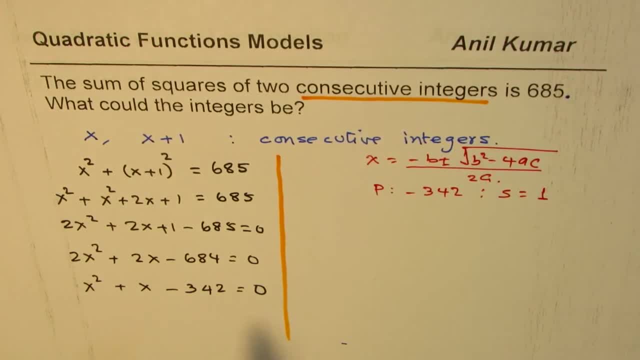 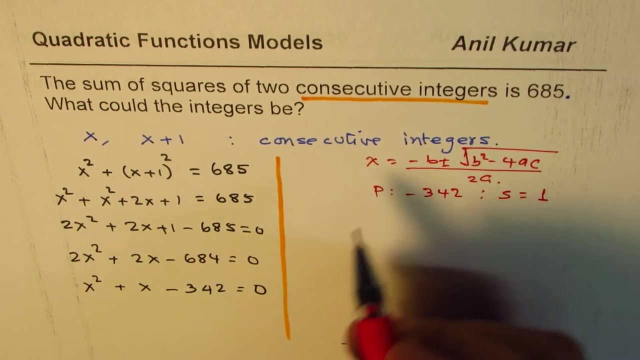 So 18.5 I get. So you're looking for two numbers which are kind of consecutive integers, right? So you're looking for two numbers which are kind of consecutive integers, right? 18 and 19 works for you, because then you get 8 times 9 is 72, right? So try these numbers. 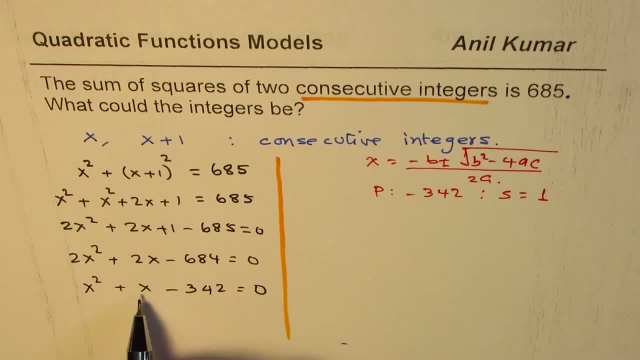 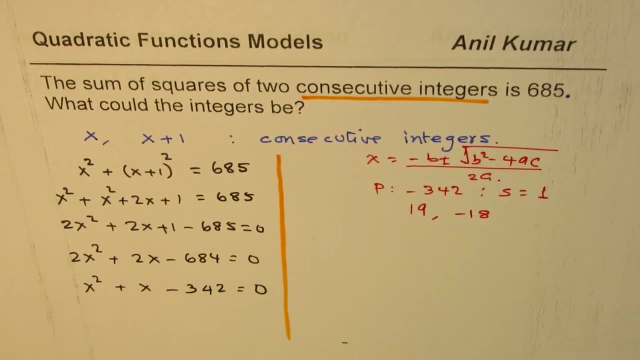 Now one of them has to be negative. The positive one is bigger number. So we'll do 19 and we'll do minus 18.. Do you see that? Okay, let's multiply 18 and 19. So we get: 18 times 19 is 342.. Perfect. 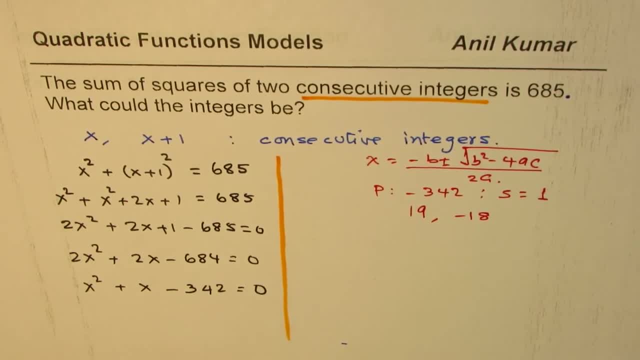 I hope you loved this idea of finding the two numbers for this right. So, using this method, I'm using product and sum. We could write this in factored form as x plus 19 times x minus 18 equal to 0, okay, So we get.